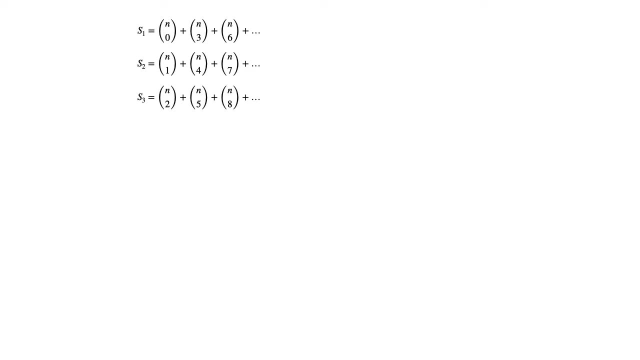 n choose 2 plus n choose 5 plus n choose 8, and so on. First let me clarify what is meant by the three dots or ellipses. It means we go as far as possible in the sequence where the last term, n choose r, is such that r is less than or equal to n, Or in other words, 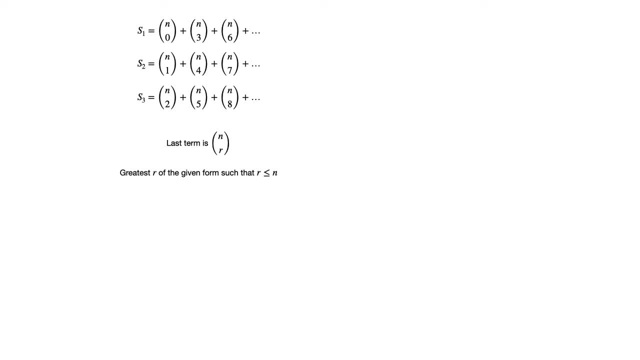 r does not exceed n. For instance, in the case of S1, each r is a multiple of 3, and so the last term will have an r value that is the largest multiple of 3 that is less than or equal to n. Similarly, 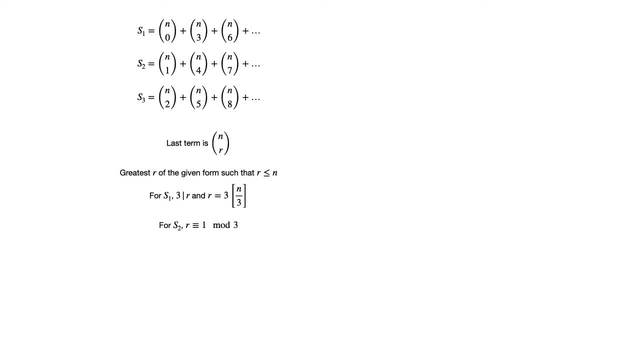 in S2, each r value is 1 more than a multiple of 3.. We stop at the largest r value of this form that does not exceed n. The same is true for S3.. The object of this video is to show that the following formula is true, Namely: Si equals. 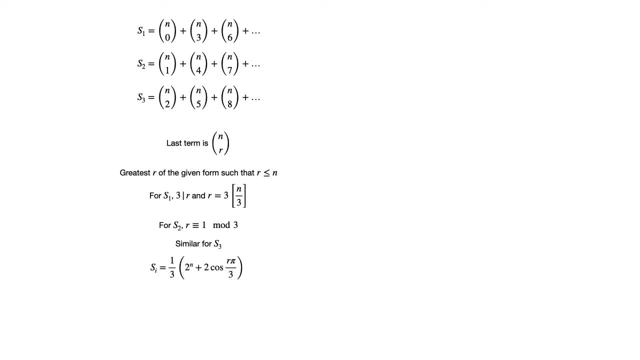 a third of 2 to the power 3.. n plus 2 cosine r pi by 3, where r equals n for i equals 1, r equals n minus 2, for i equals 2, and r equals n plus 2, for i equals 3.. 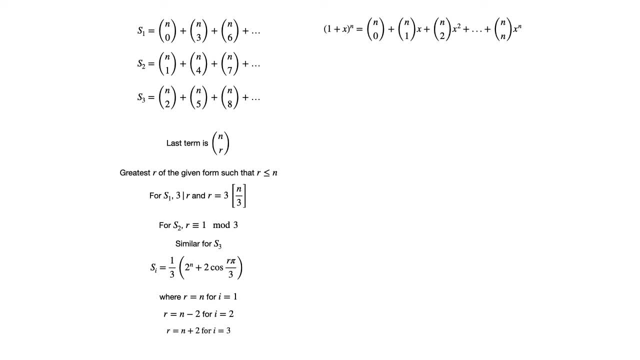 Taking our first steps, let us recall the familiar expansion for 1 plus x to the power n using the binomial theorem. Now we shall proceed by substituting in different values for x and noting the weightless expansions we obtain. For x equals 1, the expansion collapses. 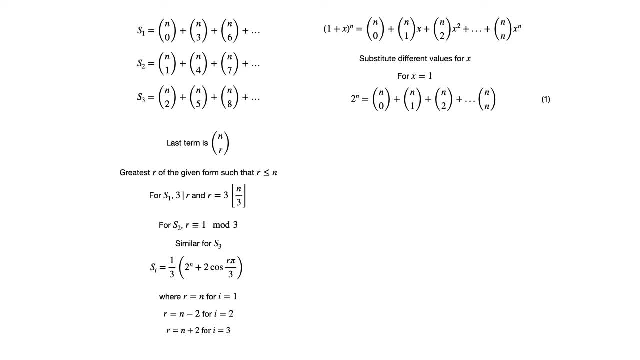 to the familiar identity S3. you surprised me… I told you. I wondered what it is. Let me show you. We difficultly realized: x equals 1.. Where is the real range for this quant Liebe from the as the sum of binomial coefficients in the nth row of Pascal's triangle, We call this equation. 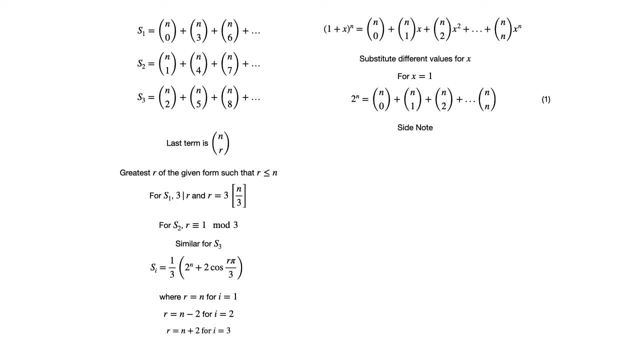 1. Before going any further, let me raise a side note. Taking our q from the theory of complex numbers and the complex cube roots of unity, we define omega as being negative half plus root 3 by 2i. In so doing, we realize that omega is one of the two complex cube roots of unity. 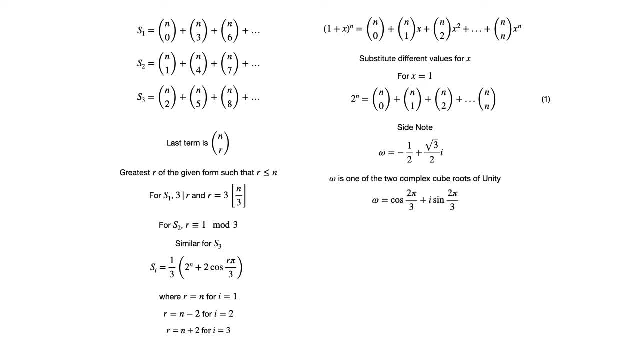 By unity we mean the number 1.. Omega can also be expressed as cosine 2pi by 3 plus i sine 2pi by 3.. For this representation we have just switched to using polar coordinates and have made use of the fact that the argument of omega is 2pi by 3. We will make frequent use of both. 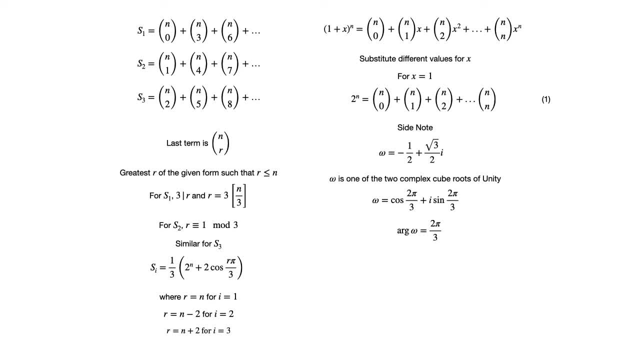 the expressions for omega throughout the course of the solution, as both will aid our calculations. Now, the second complex cube root of unity is negative, half minus root 3 by 2i, which is the complex conjugate of omega, as can be seen from this diagram of the three cube roots of 1.. 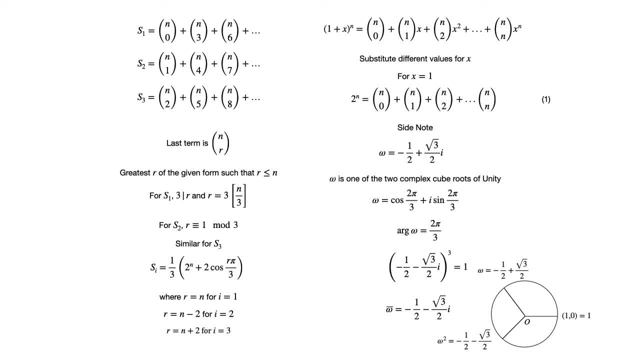 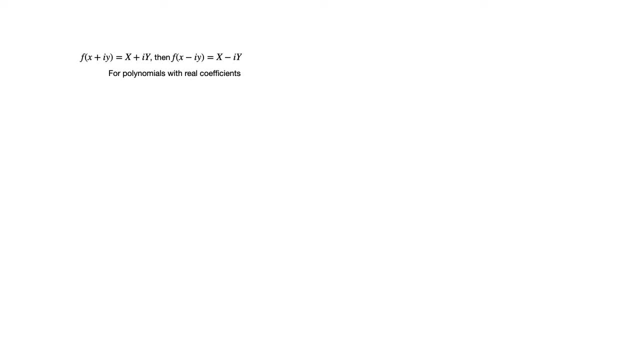 The reason the second complex cube root of unity appears as the conjugate of omega is for the simple reason that complex roots to polynomials with real coefficients are found in pairs both having identical real components and imaginary components with opposite signs. To be more specific, the three cube roots of unity, complex or otherwise, are solutions to 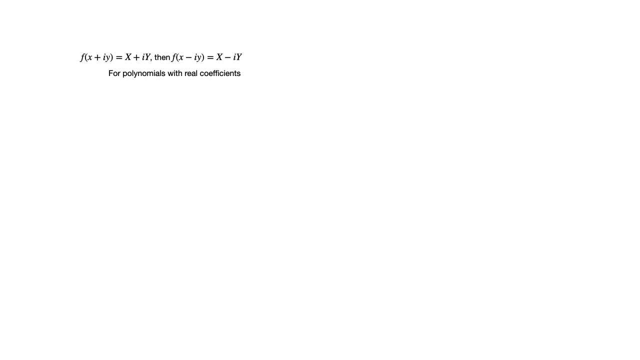 polynomial x cubed minus 1.. Indeed, this equation has degree 3, and the fundamental theorem of algebra states that it should have at most three distinct roots. This equation has exactly three of them. Factoring the expression on the left hand side, we are left with two factors. 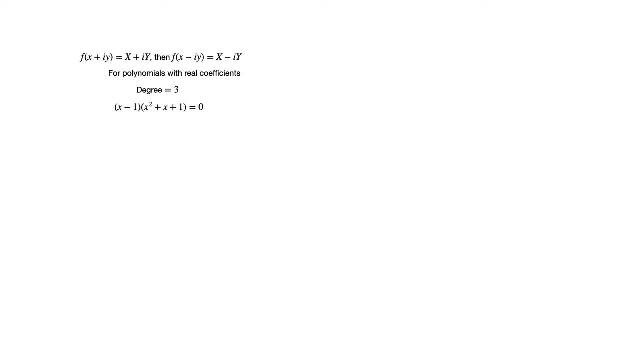 one linear and one quadratic, That is x minus 1, into x squared plus, x plus 1 equals 0.. The solution to x minus 1 equals 0 is x equals 1, which is the only real root. The solution to x squared plus x plus 1 equals 0,. 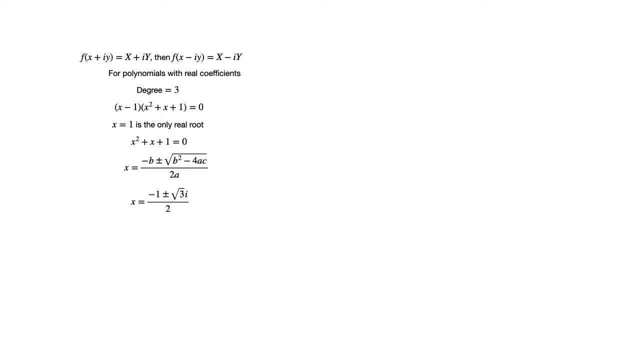 yields omega and its conjugate. Interestingly enough, the conjugate of omega is omega squared. Proving this is simplicity itself. We know that omega into omega squared equals 1 by the definition of omega as a complex cube root of 1.. So that gives us omega squared. 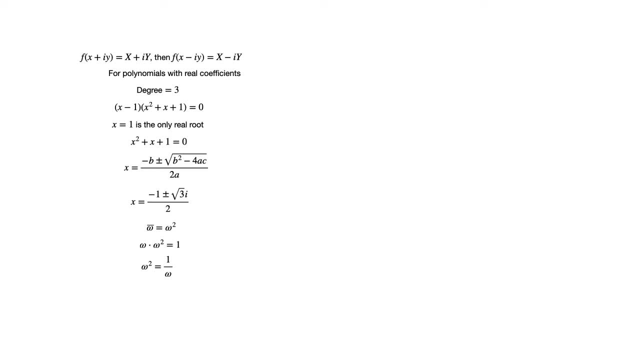 equals the reciprocal of omega. However, omega, into its conjugate, equals the modulus of omega squared, which equals 1.. The reason the modulus of omega equals 1 is since omega is a complex cube root of 1.. When we cube its modulus, the result must necessarily be 1.. In addition, 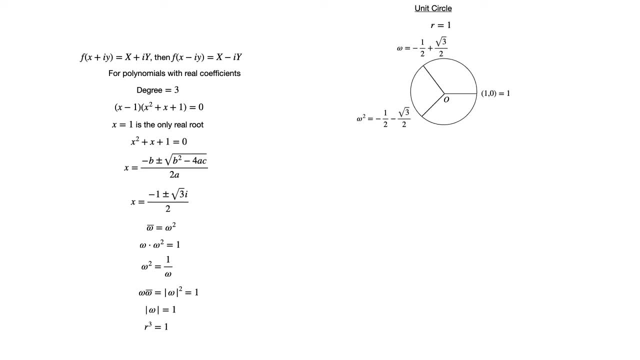 omega lies on the unit circle in the complex plane. That is another testament to the fact that its modulus should be 1.. With that preliminary, out of the way we have the statement. the conjugate of omega equals the reciprocal of omega. This quickly leads to the result that 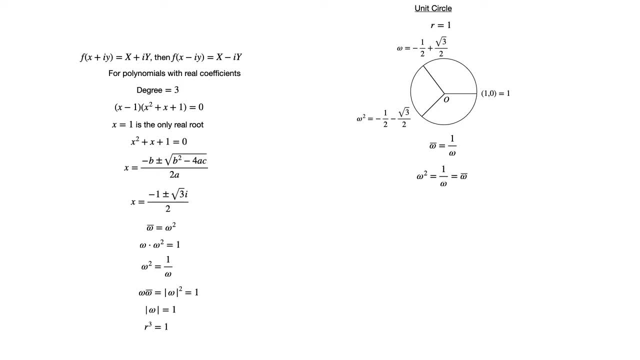 omega squared, which equals the reciprocal of omega, also equals the conjugate of omega. We can also see that omega squared equals the conjugate of omega By the fact that 4pi upon 3 equals 2pi minus 2pi by 3. This gives omega squared equals. 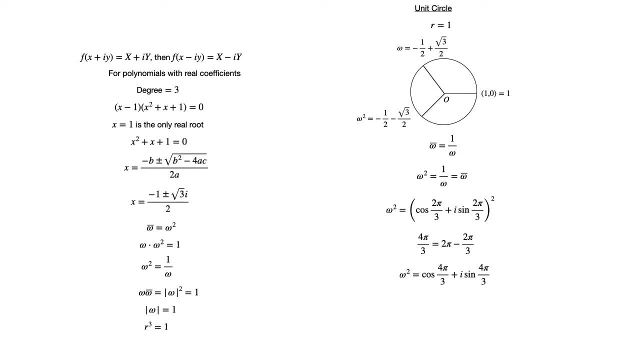 cosine 4pi by 3 plus i sine 4pi by 3, which simplifies to cosine 2pi by 3 minus i sine 2pi by 3.. This is since two angles that add up to 2pi have the same cosine values, while 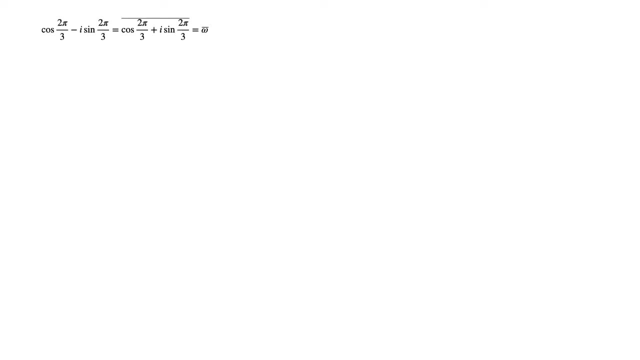 having sine values that are negatives of each other. This expression is precisely the complex conjugate of omega. Some more important facts are that omega squared squared equals omega 4, which equals omega, and 1 plus omega plus omega squared equals 0.. The first relation is: 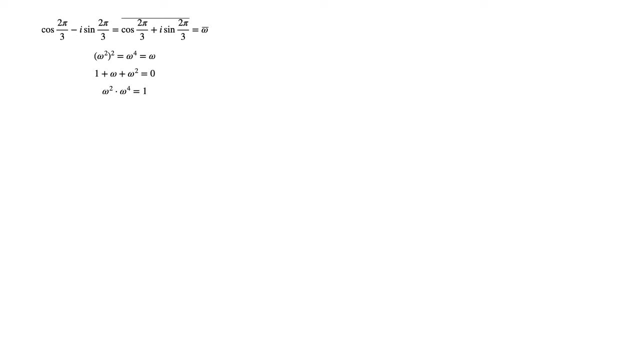 easily verified by the fact that omega squared into omega to the power of 4 equals 1.. This translates to omega to the power of 4 equals the reciprocal of omega squared, which equals omega, as was shown before. The second statement arises from the fact that omega satisfies. 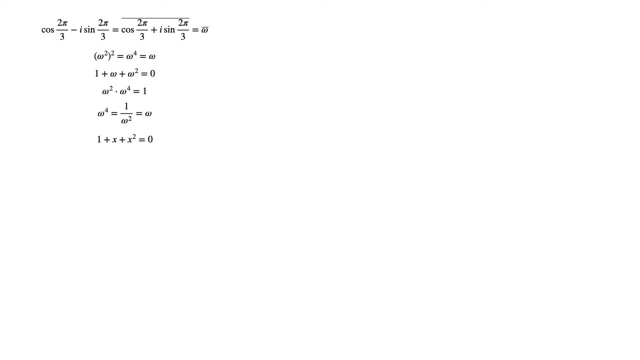 the equation 1 plus x plus x squared equals 0.. Since omega minus 1 is certainly equal to 0, it is certainly not 0.. For that matter, omega squared satisfies the same condition and hence 1 plus omega squared, plus omega to the power of 4 equals 0 as well. 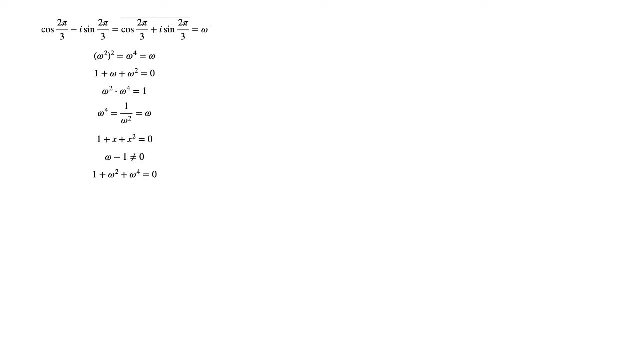 With this revision of the theory of complex numbers complete, we are ready to return to our problem that has patiently awaited us for a while now: Going back to the binomial expansion for 1 plus x to the power n and replacing x with omega and omega squared respectively. 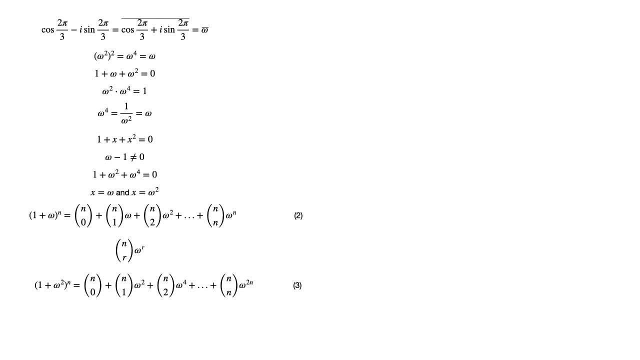 we are left with equations 2 and 3. Reading the first one out, it says: 1 plus omega to the power n equals n choose 0 plus n choose 1 omega plus n choose 2 omega squared, and so on, the last term being n choose n omega to the power n. Notice that the general 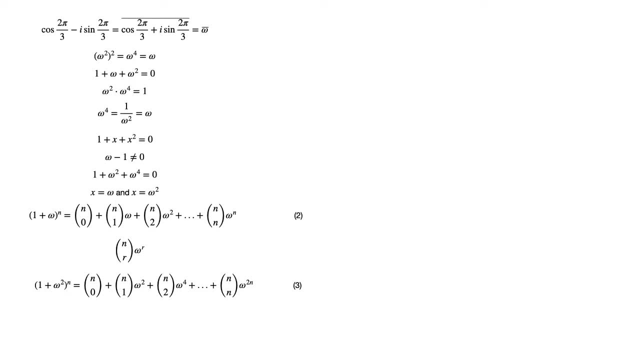 term is of the form n choose r omega to the power r. Likewise, the second one says: 1 plus omega squared to the power n equals n choose 0 plus n choose 1 omega squared plus n. choose 2 omega to the power 4, all the way up to n choose n omega to the power 2n. Here the general. 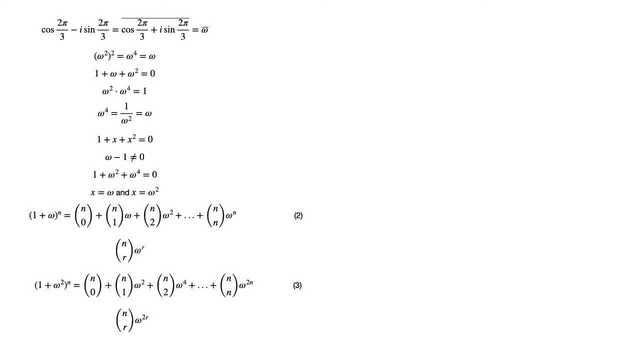 term is of the form n choose r omega to the power 2n. Here the general term is of the form n: choose r omega to the power 2n. Here the general term is of the form n choose r 2r. Adding equations 1, 2 and 3 and studying the characteristics of the general term, we 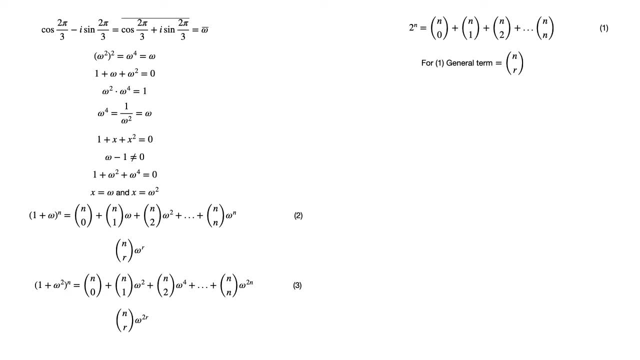 discover numerous simplifications. Commencing our analysis, we see that n choose r is a common factor in each of the general terms and is one that we shall pull out. Inside. we get the expression 1 plus omega to the power r plus omega to the power 2r. This has 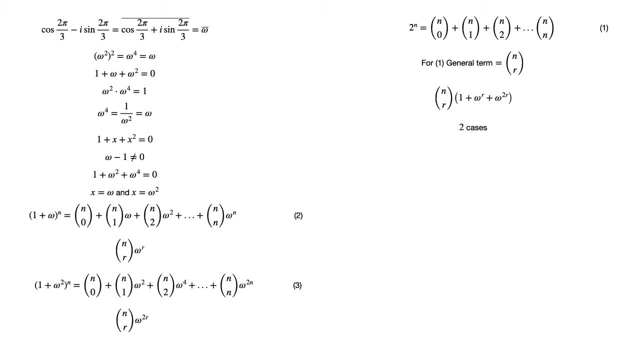 to be broken down into two cases. to find its value depending on r. The first case is where r is not a multiple of 3.. In that case, taking stock of the division algorithm, we can write the equation: r equals 3j plus m, where m is either 1 or 2, but not 0. In either case, omega. 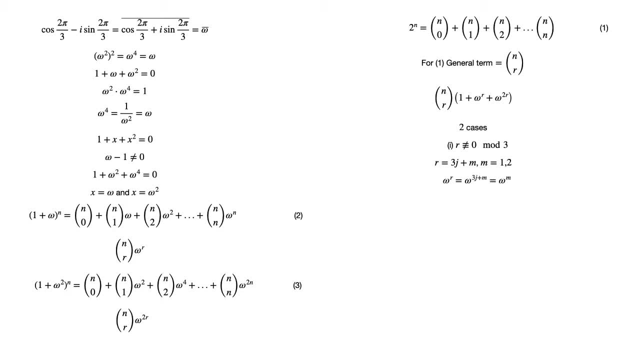 to the power r equals omega to the power 3j plus m, which equals omega to the power m, since omega raised to any multiple of 3 will yield 1, as that is the very definition of omega. If m equals 1, 1 plus omega to the power r plus omega to the power 2r equals 1.. This 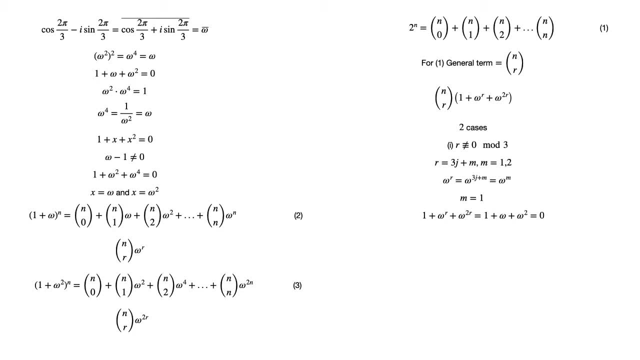 means that r equals 1 plus omega plus omega squared, which equals 0,. as was discussed earlier, If m equals 2, the expression simplifies to 1 plus omega, squared plus omega to the power 4, which also equals 0, since omega to the power 4 equals omega In both cases, m being 1 or. 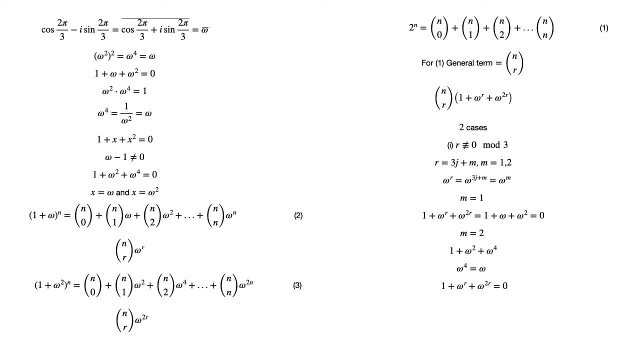 2,. 1 plus omega to the power, r plus omega to the power, 2r equals 0.. In the case that r is a multiple of 3, we have that 1 plus omega to the power, r plus omega to the power. 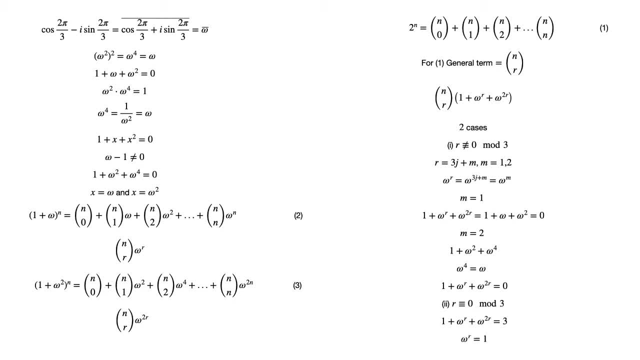 2r equals 0. Thus, m is not an aircraft. All the functions that we have to find out are the following: 3, because omega to the power, r equals 1.. After simplifying as much as we can, we see: 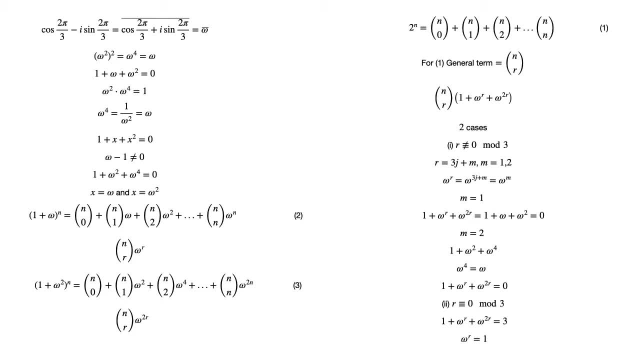 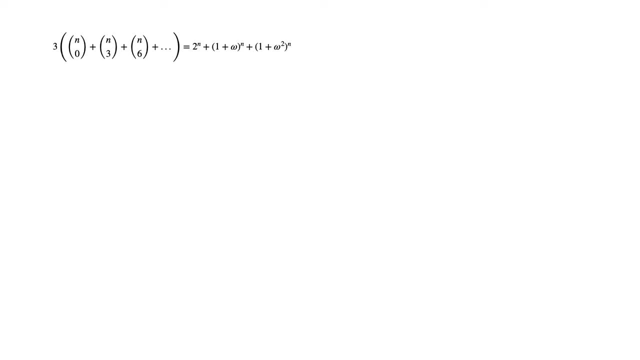 that the summation of equations 1, 2 and 3 gives us the following expression: 3 into n choose 0 plus n choose 3 plus n choose 6, and so on, which equals 2 to the power n plus 1 plus omega to the power n plus 1 plus omega, squared to the power n, The expression inside. 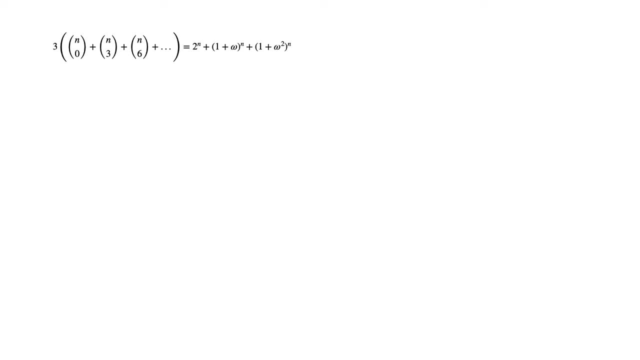 the parentheses on the left hand side should be familiar to us, as it is nothing but S1.. Great results, since the only terms that survive are those where r is a multiple of 3.. All the rest, cancel out to 0.. We will now endeavour to obtain closed form expressions of 1 plus. 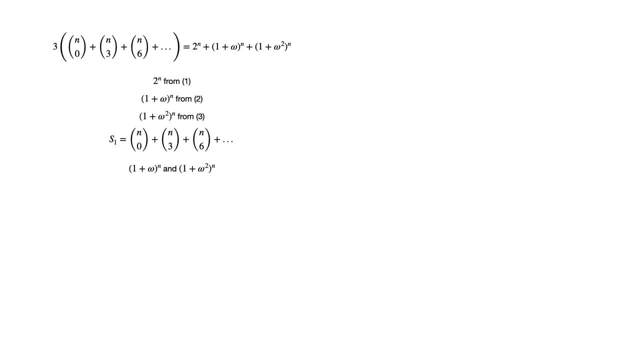 omega to the power n and 1 plus omega squared to the power n, which are members of the right hand side. We see that 1 plus omega equals 1 plus cosine, 2 pi by 3 plus i sine 2 pi by 3.. Here we make use of two well-known trigonometric identities. on RH. 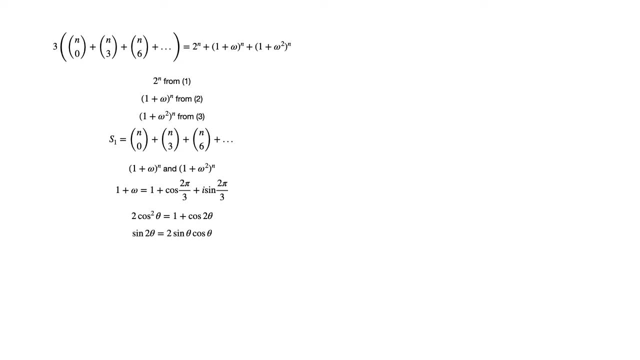 The first relates cosine theta to cosine 2 theta. It says that 2 cosine square theta equals 1 plus cosine 2 theta. Similarly, we also use the identity for sine 2 theta. Putting it all together, we obtain 1 plus omega equals 2 cosine squared pi by 3 plus i into 2 sine pi by 3 cosine. 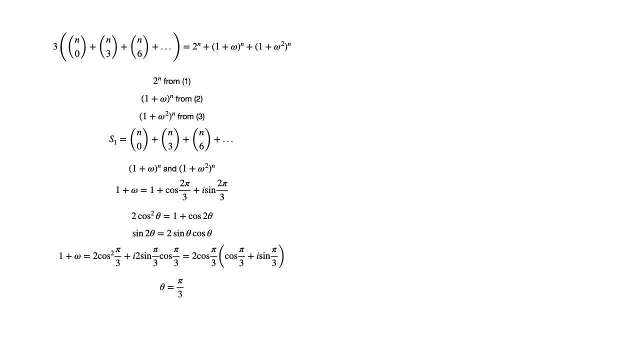 pi by 3, which equals 2 cosine pi by 3, into cosine pi by 3 plus i sine pi by 3.. The common factor to cosine pi by 3 is factored out. Those of you with a sharp memory will remember. 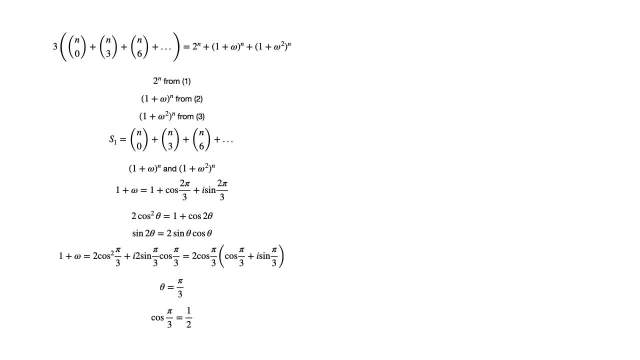 that cosine pi by 3 equals a half. Therefore the RHS simplifies to cosine pi by 3 plus i sine pi by 3.. Upon raising both sides to n and applying De Moivre's theorem, we have 1 plus omega to the power. n equals cosine n pi by 3 plus i sine n pi by 3.. In like manner, 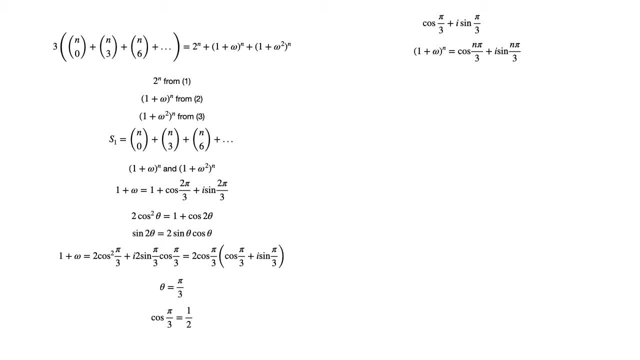 we obtain the closed form expressions for 1 plus omega, squared to the power n. A similar equation is used for the cosine pi by 3 equation. We obtain the closed form expressions for 1 plus omega, squared to the power n. A similar equation is used for the cosine pi by 3 equation. 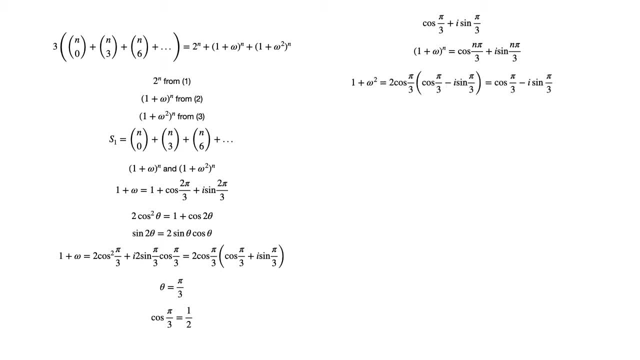 Another analysis to the previous case yields the result: 1 plus omega squared equals 2 cosine pi by 3 into cosine pi by 3 minus i sine pi by 3.. Notice how 1 plus omega squared is the complex conjugate of 1 plus omega, just as omega squared is the conjugate of omega. The 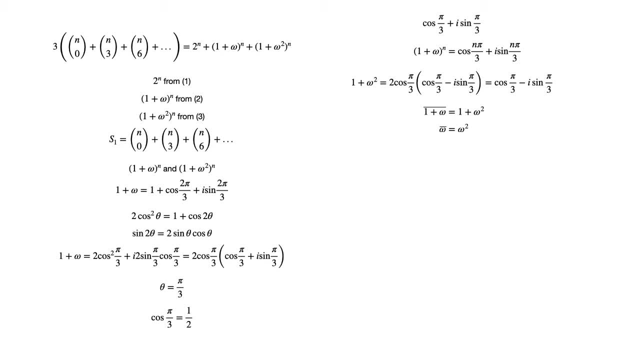 justification of this fact is trivial: The same real number is getting added to both omega and omega squared, while the imaginary components remain unchanged, and so the fact that they are negatives of each other still remains unchanged. Raising the expression for 1 plus omega squared to the power n, we find that it equals cosine. 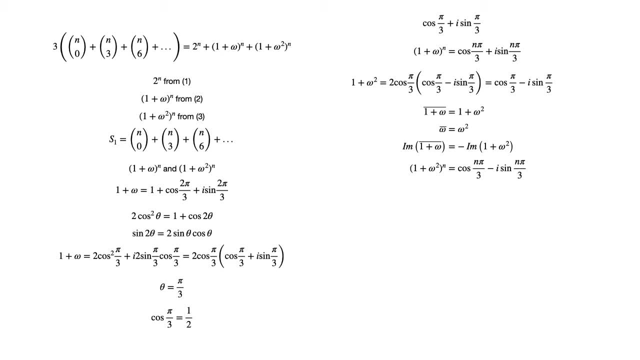 n pi by 3 minus i sine n pi by 3.. Adding 1 plus omega to the power n to 1 plus omega squared to the power n, we find that the sine terms cancel out, as they have opposite sines. The cosines have equivalent arguments and so combine with a coefficient of 2. Thus the 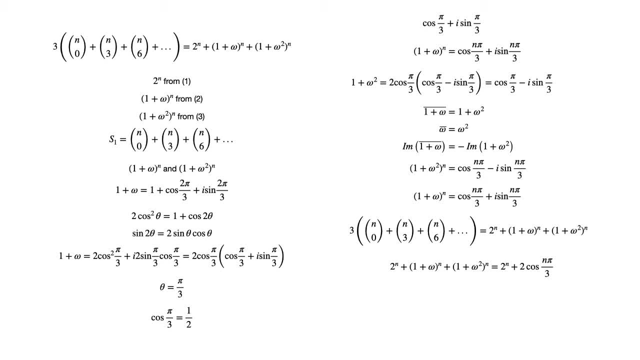 right hand side of the equation produced by the summation of equations 1,, 2 and 3 gives us 2 to the power n, plus 2 cosine pi by 3.. This is the sum of the equations 1,, 2 and. 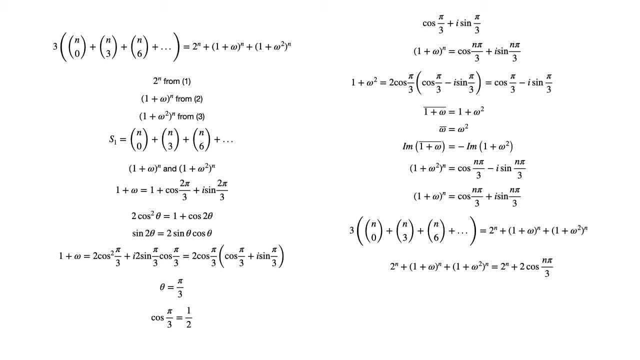 3. The final and easiest step that now remains is to switch the 3 over to the other side of the equation to get it into the form that we desire. Doing this, we have s1- equals n. choose 0 plus n, choose 3 plus n, choose 6, and so on: equals. 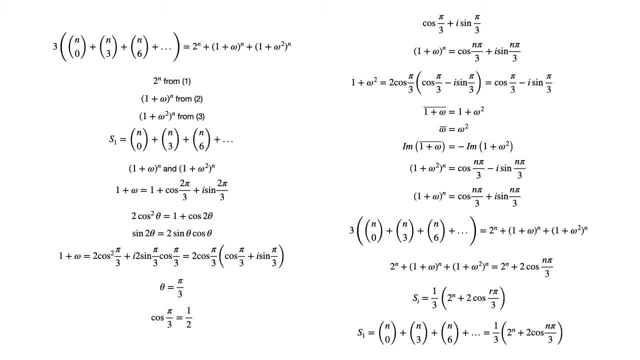 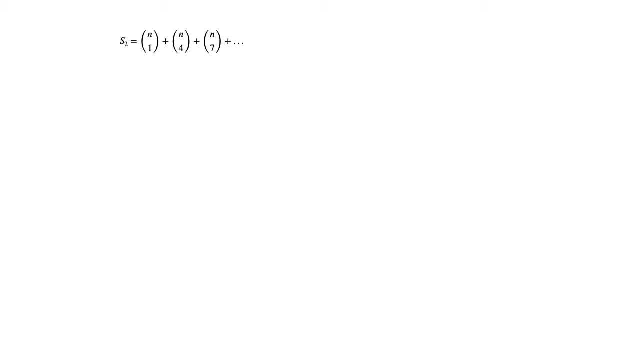 a third of 2 to the power n plus 2 cosine n, pi by 3, which is exactly what we sought out to prove. With the case for s1. shown to be true, we now turn our attention to s2.. We apply similar principles as we did in the case of s1 to arrive. 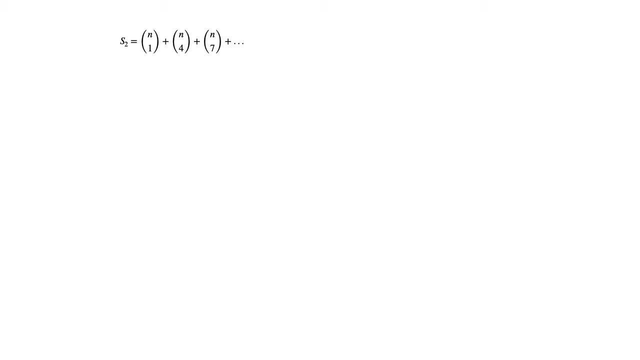 at our answer. It should be noted that now all the hard work that the problem demands has been completed in computing s1 and all that is left is some simple algebraic manipulation to drive the problem home. Continuing our journey, we now compute omega squared into. 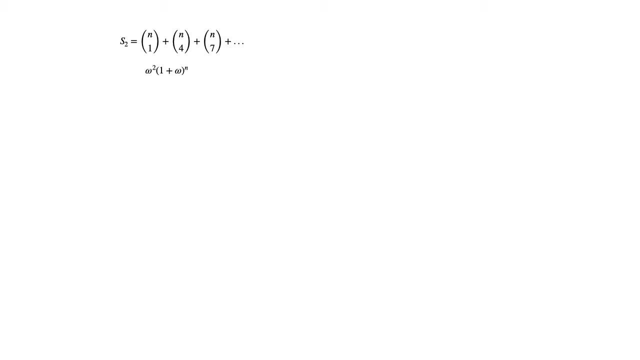 1 plus omega to the power n, which we name equation 4, by multiplying equation 2 by omega squared. Then we calculate omega into 1 plus omega squared to the power n, by multiplying equation 3 by omega. This is named equation 5.. Equations 2 and 3 were defined earlier. 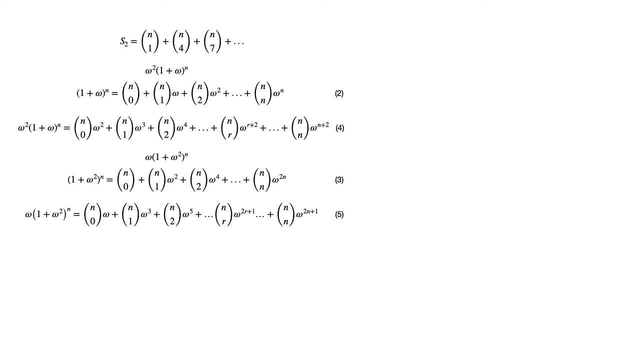 in the video. Again, looking at the general terms, we notice that for equation 4, it takes the form n choose r omega to the power r plus 2, and for equation 5, it takes the form n choose r omega to the power 2r plus 1.. Once we add equations 1,, 4 and 5, only those terms. 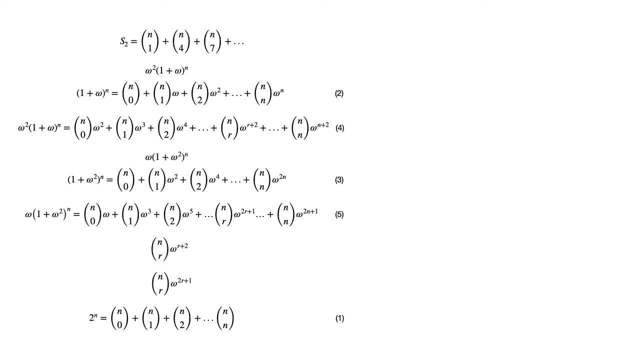 survive that are incorporated in S2.. Indeed, we find that the general term takes the form n choose r into 1 plus omega to the power r plus 2 plus omega to the power 2r plus 1.. Observe how we can write omega to the power 2r plus 1 as omega to the power 2r plus 4. 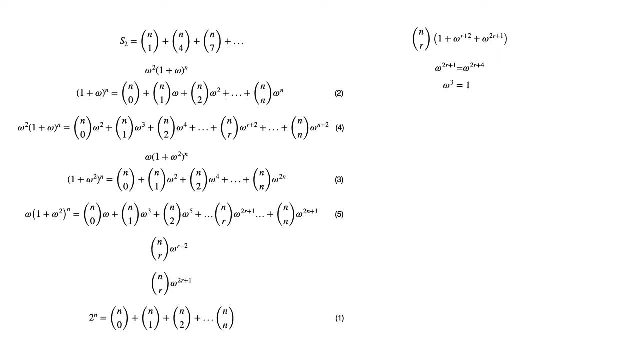 owing to the fact that omega cubed equals 1.. This gives us the expression 1 plus omega to the power r plus 2 plus omega to the power 2r plus 1.. If r plus 2 is not a multiple of 3, or in other words r is not congruent to 1 mod 3,. 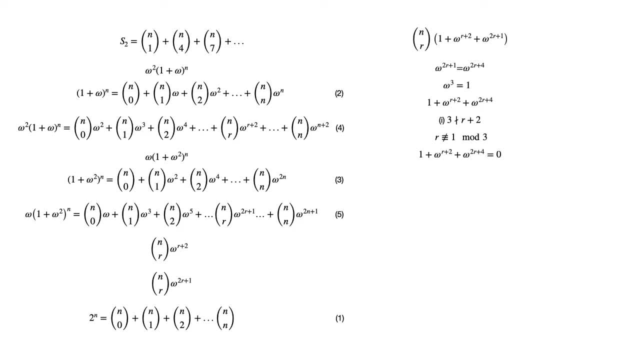 the expression in the parentheses simplifies to 0.. The reasoning is the same as in the case of S1.. Since applying the division algorithm to r plus 2, this time we will get a remainder m that is either 1 or 2, but not 0. This yields the expression 1 plus omega to the power m. 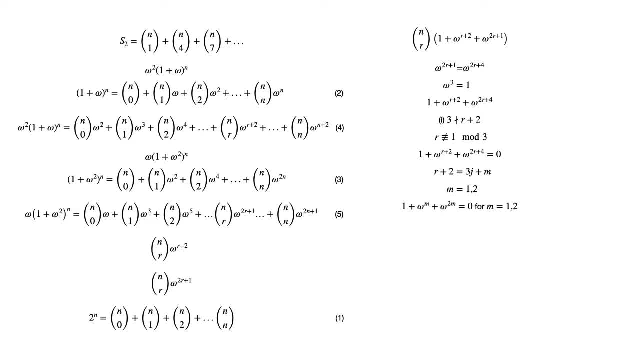 is omega to the power 2m, which was shown earlier to be 0.. When m takes on the values 1 and 2, in the case that r plus 2 is a multiple of 3, 1 plus omega to the power r plus 2 plus. 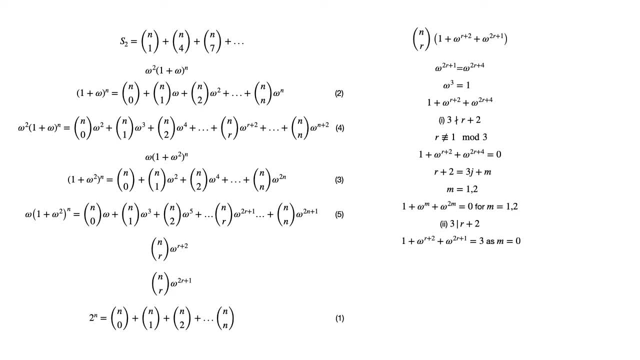 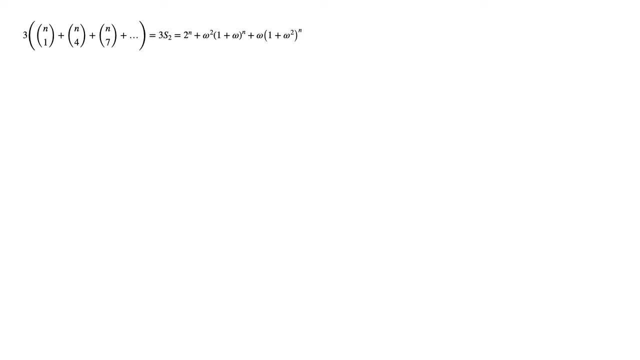 omega to the power, 2r plus 1 equals 3, as m equals 0. That is why, after adding equations 1, 4 and 5 on the left hand side, we have 3 into n choose. 1 plus n choose. 4 plus n choose. 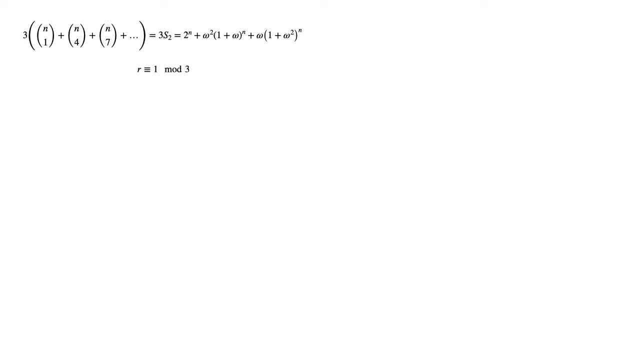 7 and so on. Only those terms where r leaves a remainder of 1 on division by 3 make it through the artificial C we have created. On the right hand side we have the terms omega squared into 1 plus omega to the power n, and omega into 1 plus omega squared to the. 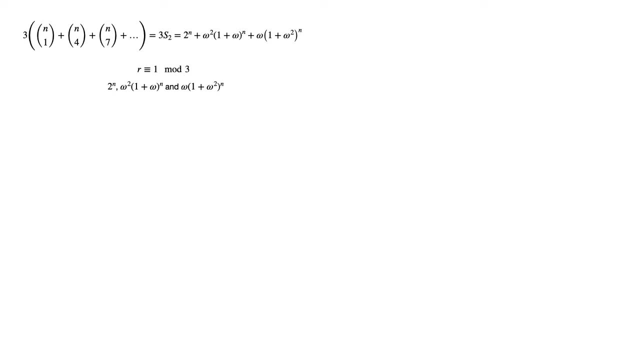 power n. Getting closed form expressions for the second and third terms mentioned should now be easier than breathing air. We have that. omega squared into 1 plus omega to the power n equals cosine 2pi by 3 minus i sine, 2pi by 3 into cosine n pi by 3 plus i sine. 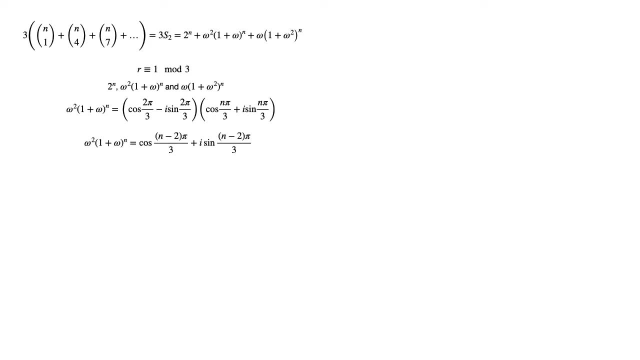 n pi by 3. Adding the arguments gives us cosine n minus 2pi by 3 plus i sine n minus 2pi by 3.. The argument for omega squared was negative: 2pi by 3. Similarly, omega into 1 plus omega. 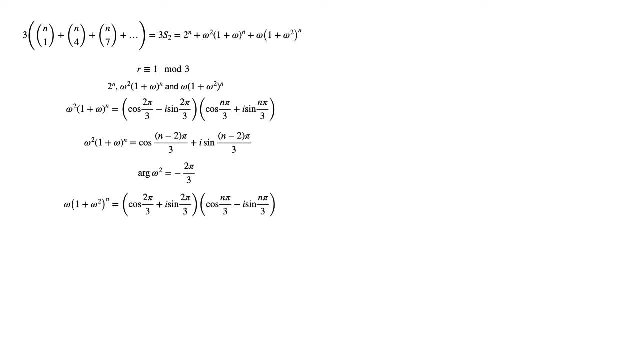 squared to the power n equals cosine 2pi by 3 plus i sine 2pi by 3, into cosine n pi by 3 minus i sine n pi by 3, which equals cosine n minus 2pi by 3, minus i sine n minus 2pi. 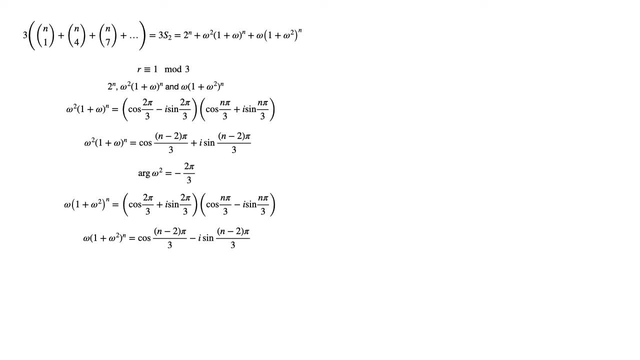 by 3.. Adding omega squared into 1 plus omega to the power n and omega into 1 plus omega squared to the power n yields 2 cosine n minus 2pi by 3.. The argument for omega squared was negative: 2pi by 3.. Similarly, omega into 1 plus omega. 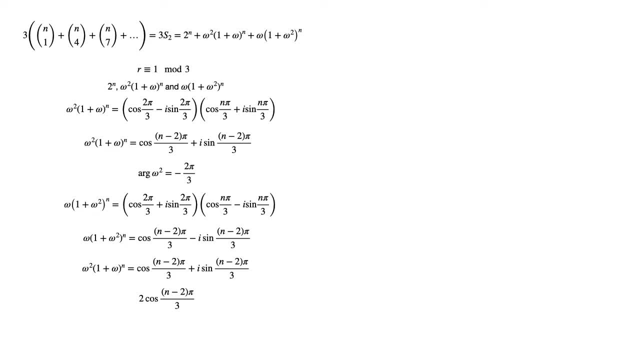 Once again, the sign terms cancel, since they are negatives of each other. Curiously, they are also the only terms contributing to the imaginary components. Compiling all our findings, we see that the right hand side of the equation, produced from adding equations 1, 4 and 5, simplifies to 2, to the power n plus 2 cosine n minus 2 pi. 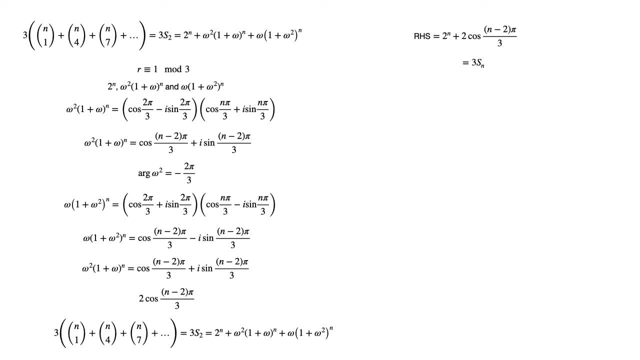 by 3, and this equals 3s2.. Lastly, the 3 is brought to the other side of the equation to match the form given in the statement of our problem. A closer investigation reveals that the formula we have established does indeed match with the one given on the first. 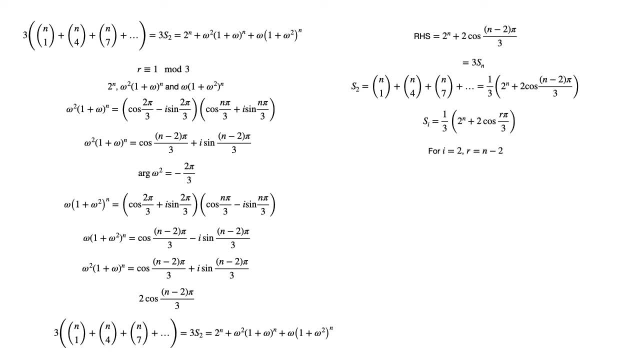 page for the case i equals 2,. more precisely, r equals n minus 2.. Finally, the case S3, which has awaited its turn long enough, comes into the spotlight In like fashion to the previous two cases, we compute two new expressions, omega, into. 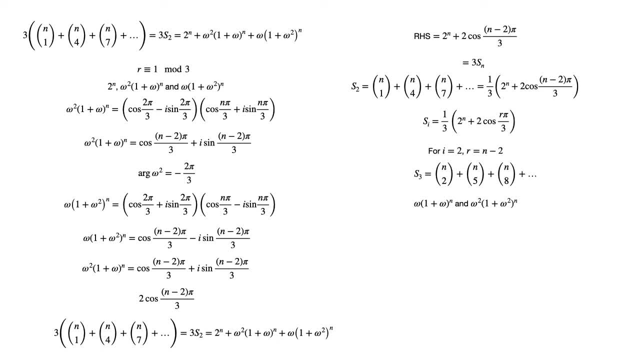 1 plus omega to the power n and omega squared. We shall call these equations 6 and 7 respectively. Equation 6 is equation 2 multiplied by omega, and equation 7 is equation 3 multiplied by omega squared. Notice how, in the case of 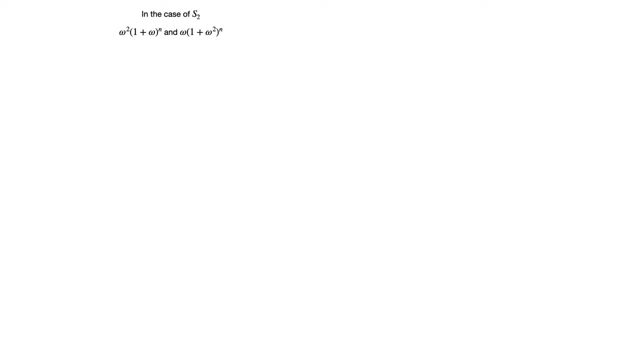 S2, we calculated omega squared into 1 plus omega to the power n and omega into 1 plus omega squared to the power n. Here we have done exactly the opposite, in the sense that equation 2 is being multiplied by omega and equation 3 by omega squared After adding. 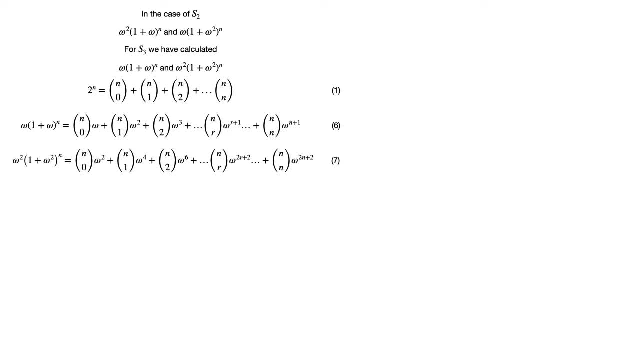 equations 1, 6 and 7, we get the following equation: Entries r into 1 plus omega to the power r plus 1 plus omega to the power 2r plus 2.. The terms that survive are those where r is congruent to 2 mod 3.. These are the terms. 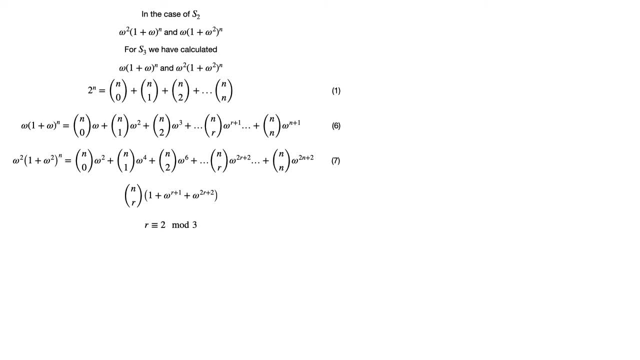 present in S3.. We can leverage this same reasoning as in the previous two cases. If r plus 1 is not a multiple of 3, it leaves a remainder m that is either 1 or 2 on division by 3.. In both cases the expression 1 plus omega to the power m plus omega to the power 2 is: 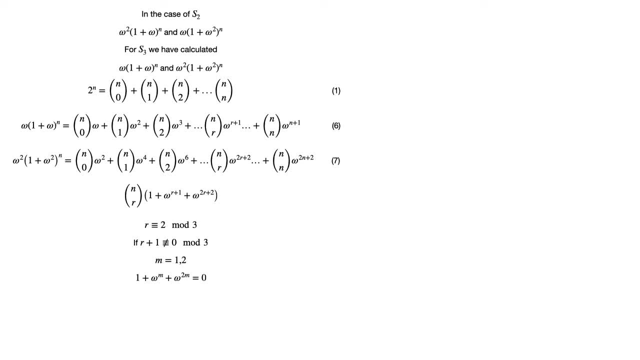 the same as in the previous two cases. In both cases, the expression 1 plus omega to the power 2m comes out to 0. In the case that m equals 0,, the expression has a value of 3.. This leaves us with equation 2 and x2 plus x5 plus x8 and so on, which equals 3s3. equals. 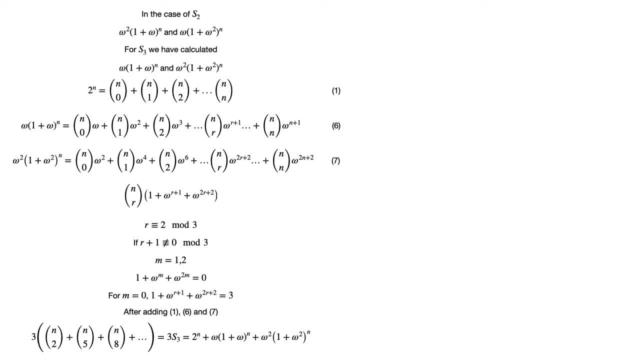 2 to the power n plus omega into 1 plus omega to the power n plus omega. squared into 1 plus omega. squared to the power m Here omega into 1 plus omega to the power n equals cosine 2pi by 3 plus i-sin 2pi by 3 into cosine n pi by 3 plus i-sin 2pi by 3 plus i-sin 2pi. 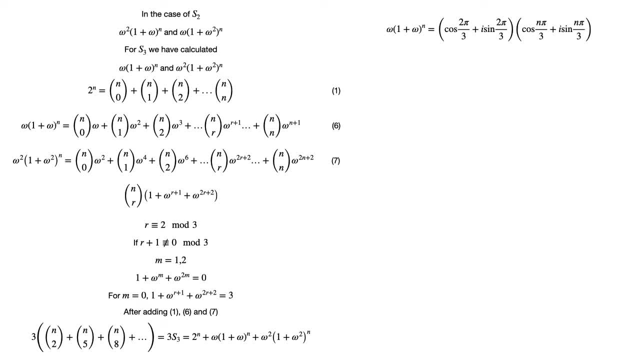 by 3 into 2pi by 3 plus i-sin 2pi by 3.. In total it gives us m equals m times m plus n pi by 3 plus i sine n pi by 3. This equals cosine n plus 2 pi by 3 plus i sine n plus. 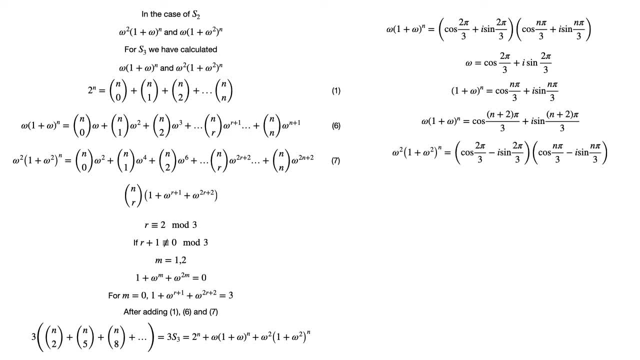 2 pi by 3.. In similar stride, omega squared into 1 plus omega squared to the power n equals cosine 2 pi by 3 minus i sine 2 pi by 3 times cosine n pi by 3 minus i sine n pi by 3.. This 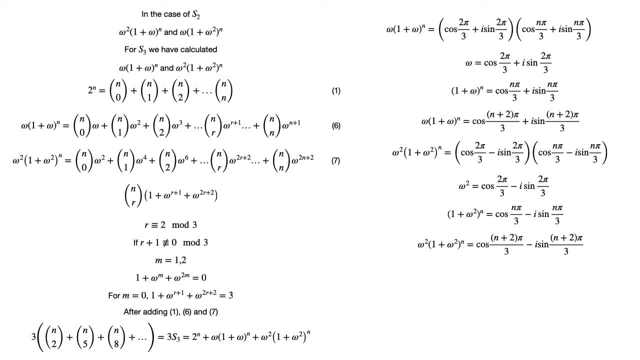 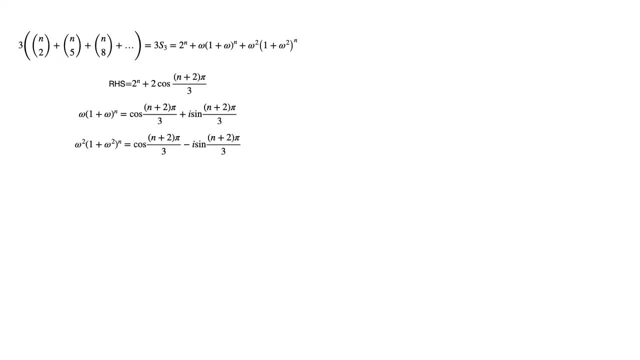 can be replaced by cosine n plus 2 pi by 3 minus i sine n plus 2 pi by 3.. Finally, the right hand side of the sum of 1, 6 and 7 condenses to 2, to the power n plus 2. cosine n plus 2. 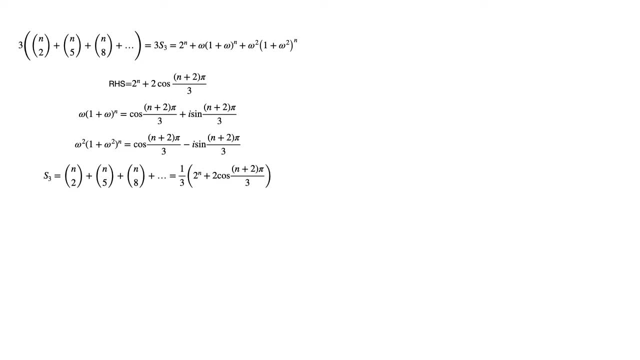 pi by 3. And moving the 3 to the other side gives S3 equals n choose 2 plus n choose 5 plus n choose 8, and so on, which equals a third of 2 to the power n plus 2, cosine n plus 2. 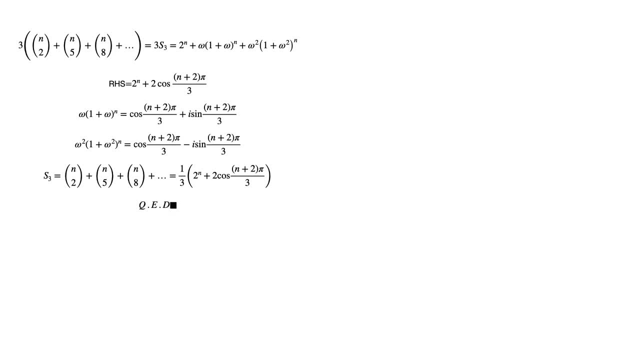 pi by 3.. With this successful computation of S3 comes the culmination of our problem, and what a remarkable one it was. This problem serves as a fine example of those cases when complex numbers rare themselves. How, one could wonder, do complex numbers help in the solution of problems posed entirely?